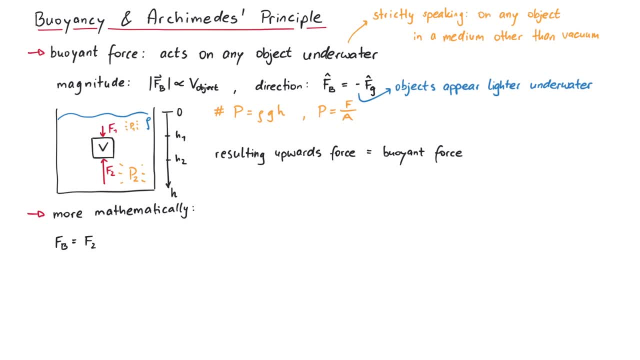 The buoyant force is defined as the difference of the force below minus the forces above works as pressure times area. so we have p2 a minus p1 a. Next, we use the hydrostatic equation to write pressure as the fluid density times, g times the 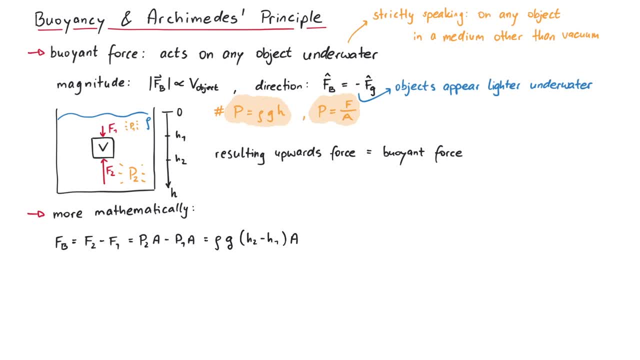 depth, where we measure the pressure common factors to the front, we can recognize the object's volume as h2 minus h1 times the area A. Here the density is a property of the fluid, the volume is a property of the object and g is a constant. Furthermore, density times volume is mass, In particular. 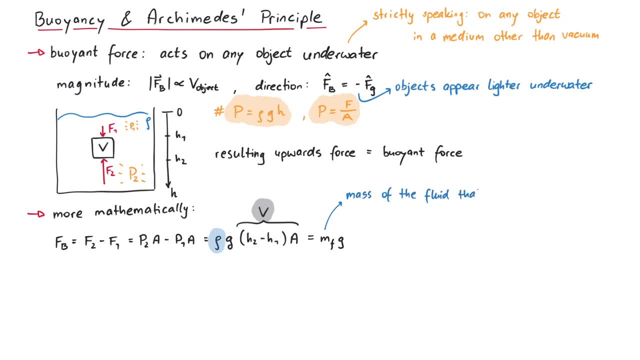 this mf denotes the mass of the fluid that would be in the volume v but is actually displaced by the object. This looks like a gravitational force. Here we already found Archimedes' principle: The buoyant force acting on an object is equal to the weight. 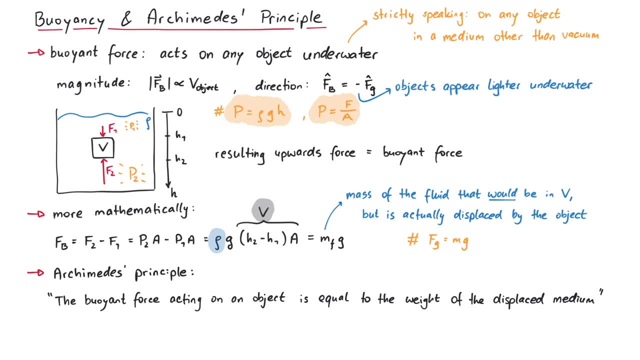 of the displaced medium. This is not only true for fluids, but for any medium. For instance, Archimedes' principle is the reason why a balloon filled with helium can float. Helium is simply lighter than the same volume of air. Finally, 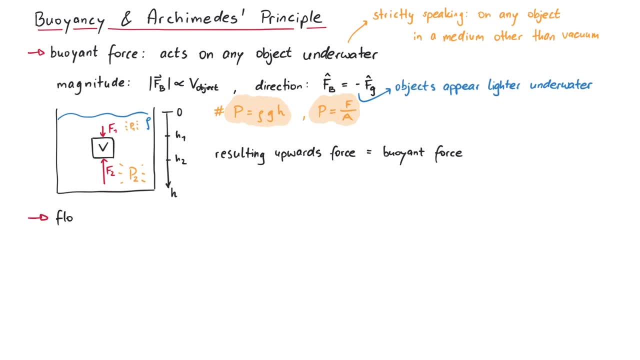 let us investigate how we can determine whether an object floats or sinks in a given medium. We will see that this is decided by the respective densities. Consider the same situation as before, where some object with density rho o is submerged in a fluid with density rho. 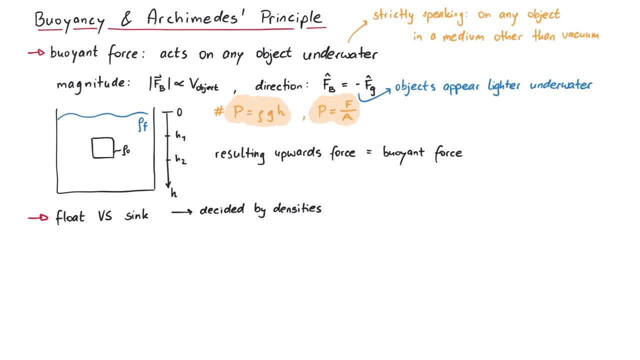 f. There are two forces acting here, the gravitational force and the buoyant force. Due to Newton's second law of motion, the acceleration of the object is equal to the buoyant force acting on an object. The velocity of the object is given by the sum of all forces, so Fb minus. 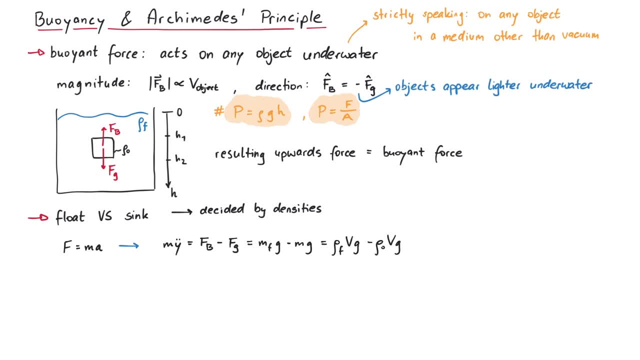 Fg. We can write this using the densities as rho f minus rho o times the volume and g. Now if rho o is larger than rho f, the acceleration is negative, therefore the object sinks down. On the other hand, if rho o is smaller than rho f, the acceleration is positive. 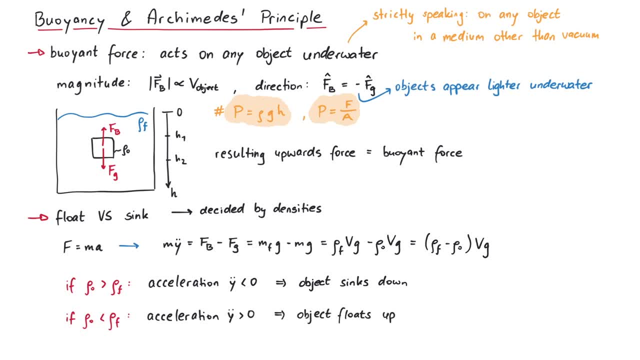 and the object floats up. And that's pretty much it for this video. Thanks for watching.